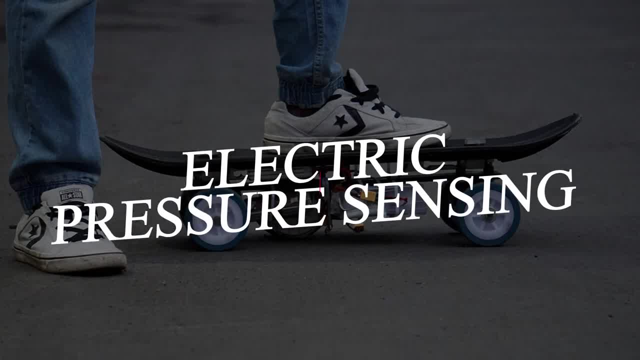 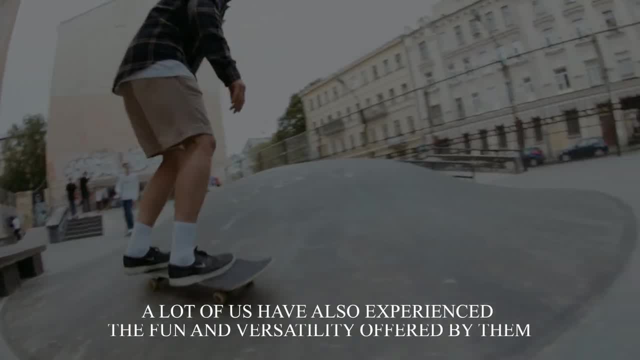 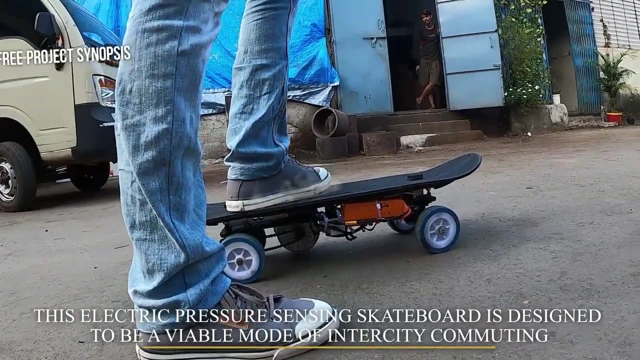 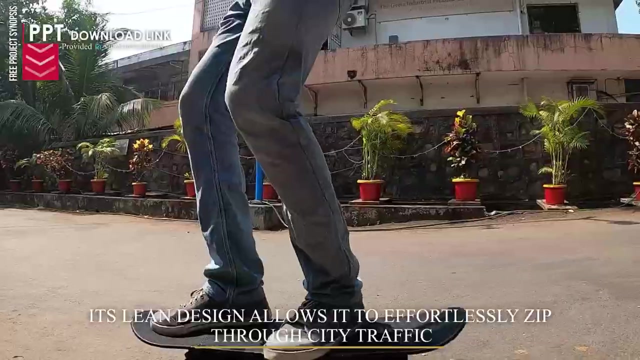 Electric Pressure Sensing Skateboard. We are well acquainted with conventional skateboards. A lot of us have also experienced the fun and versatility offered by them. This electric pressure sensing skateboard is designed to be a viable mode of intercity commuting. Its lean design allows it to effortlessly zip through city traffic. 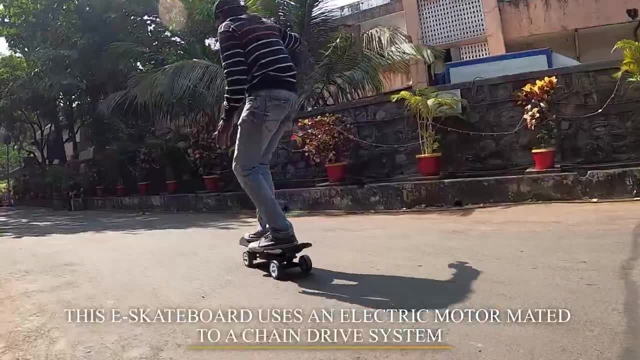 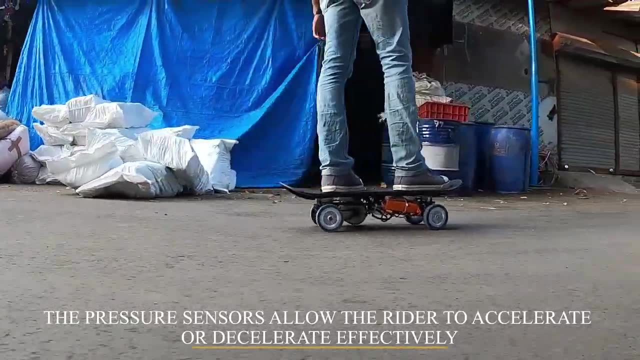 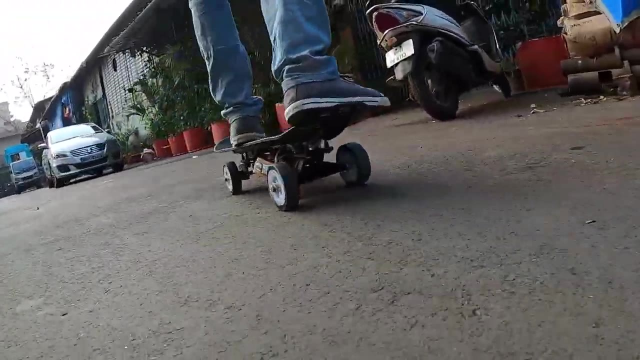 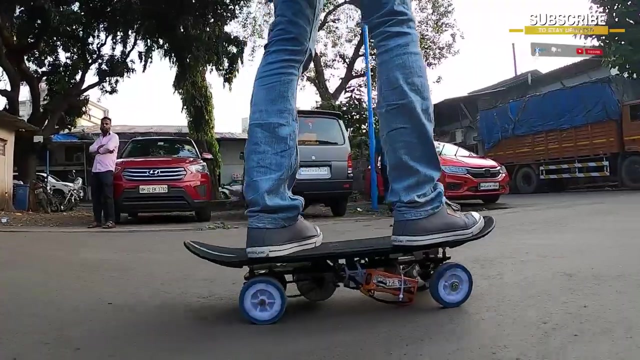 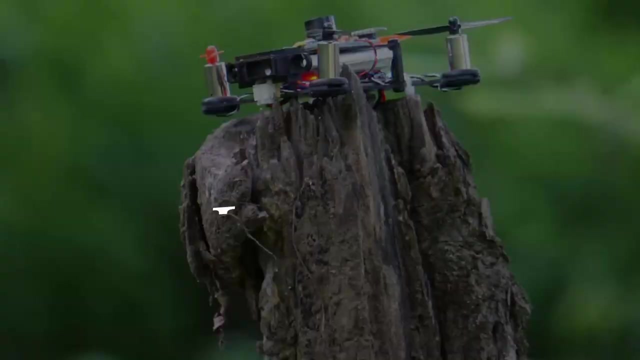 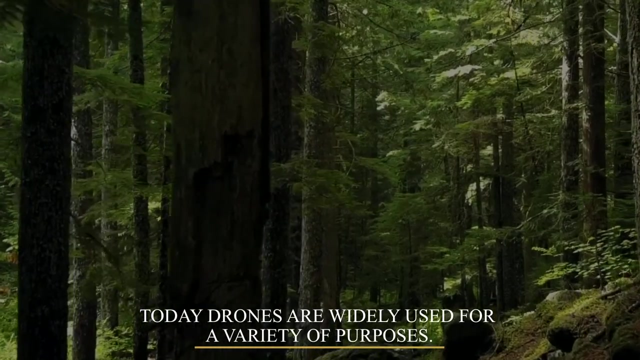 This skateboard uses an electric motor mated to a chain drive system. The pressure sensor allows the rider to accelerate or deaccelerate with ease. LiDAR Drone with Proximity Sensing. Today, drones are widely used for a variety of purposes. However, drones are costly and are highly prone to damage while flying. 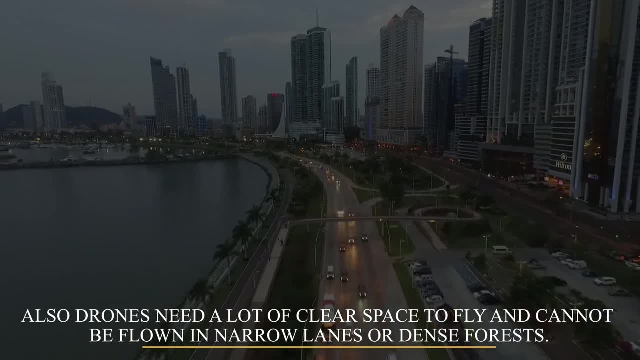 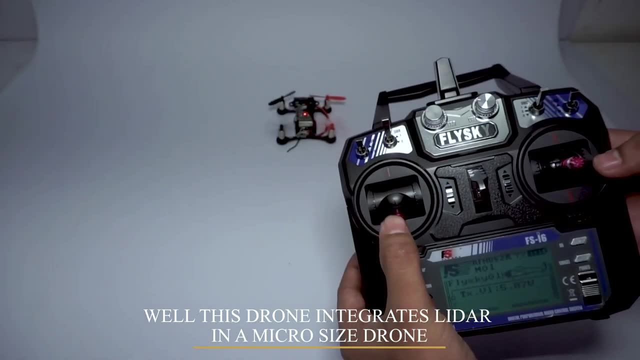 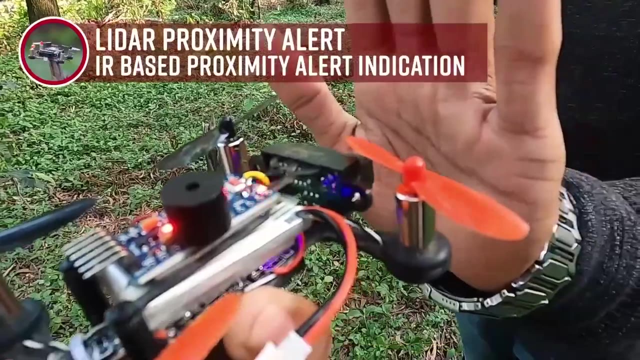 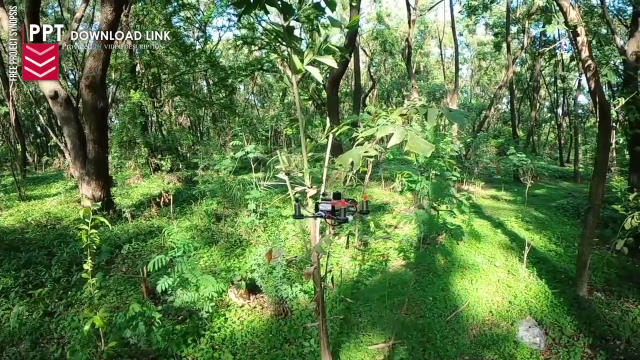 Also, drones need a lot of player space to fly and cannot be flown in narrow lanes or dense forests. Well, this drone integrates LiDAR with a micro-sized drone. This helps us study obstacle avoidance while flying in dense forests. This drone can also be used to fly in narrow lanes or dense forests or compact spaces. 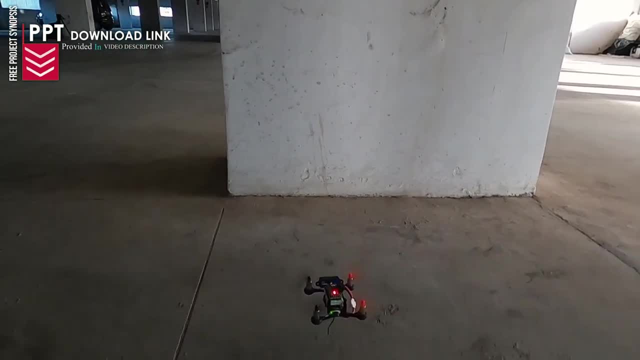 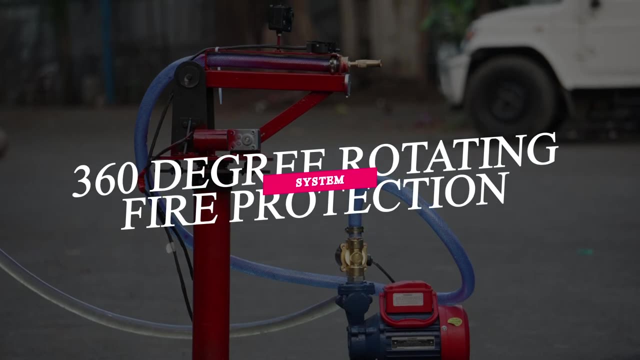 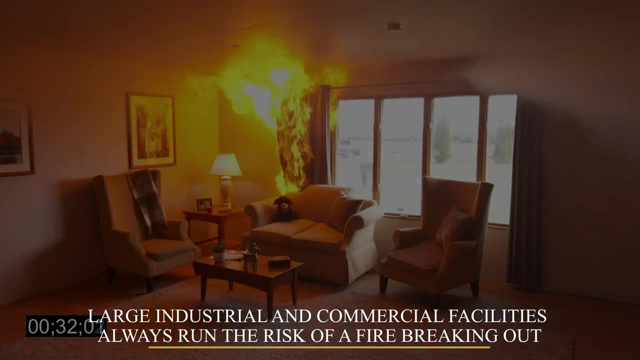 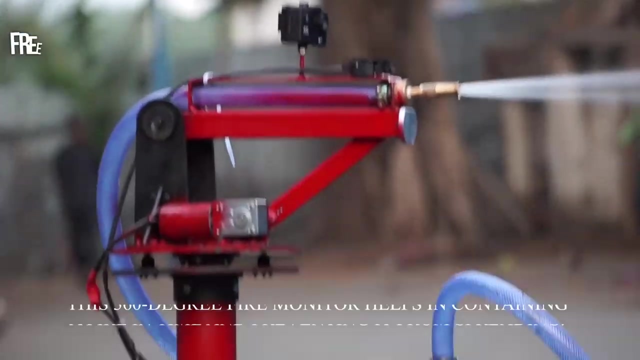 360° Rotating Fire Protection System. Large industrial and commercial facilities always run the risk of a fire breaking out. If not curbed in time, such fires could go rampant. This can lead to huge loss of life and property. This 360° fire monitor helps in containing a fire in time and preventing it from spreading. 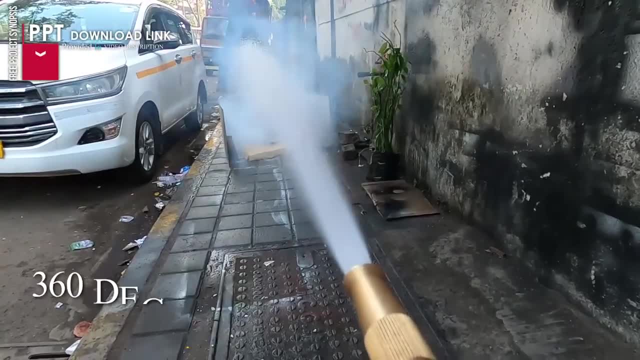 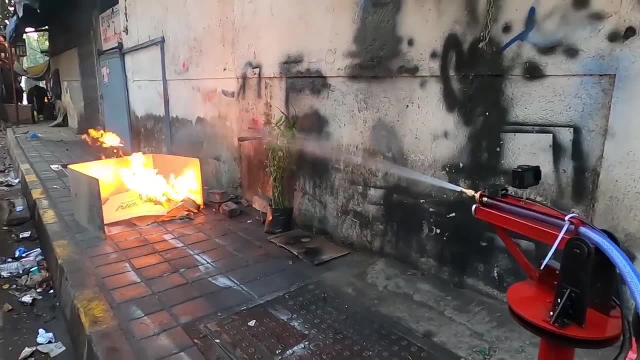 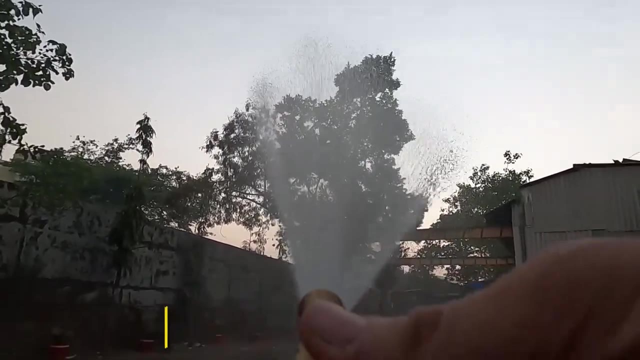 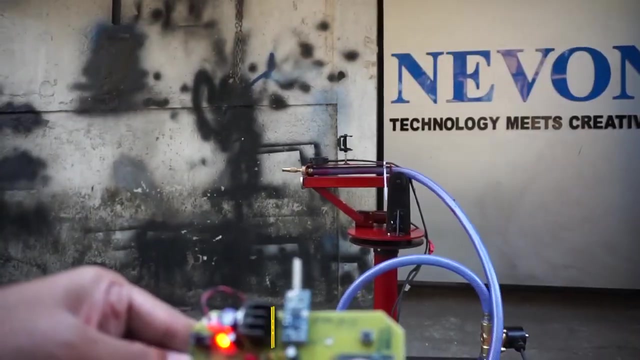 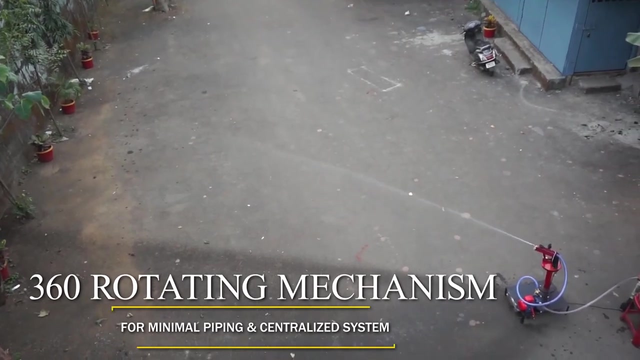 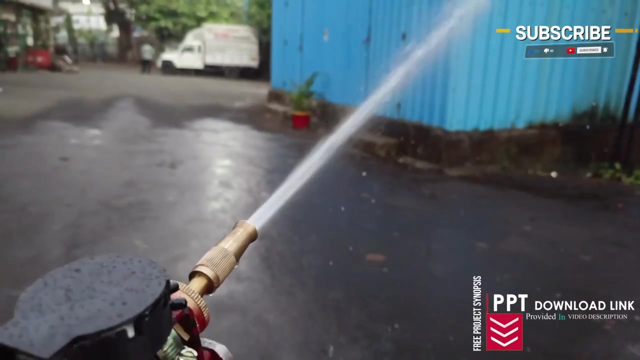 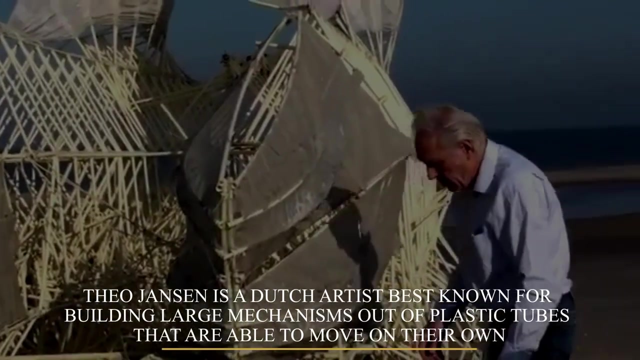 instantly. The drone can also be used to detect fire in the air. 8-Leg Spider Robot Using Theo Jensen Mechanism. Theo Jensen is a Dutch artist best known for building large mechanisms out of plastic. He is known for building large mechanisms out of plastic. 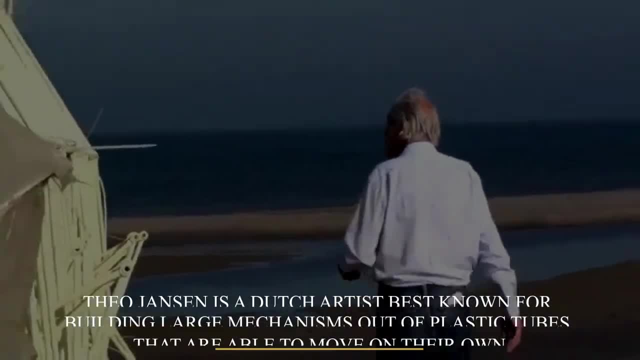 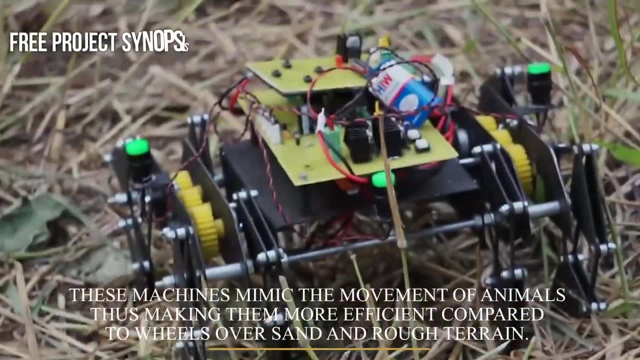 He is known for building large mechanisms out of plastic. The robot has an array of small plastic tubes and can move on its own. Heavily inspired from nature, these machines are a fusion of art and engineering. These machines mimic the movement of animals, thus making them more efficient compared to 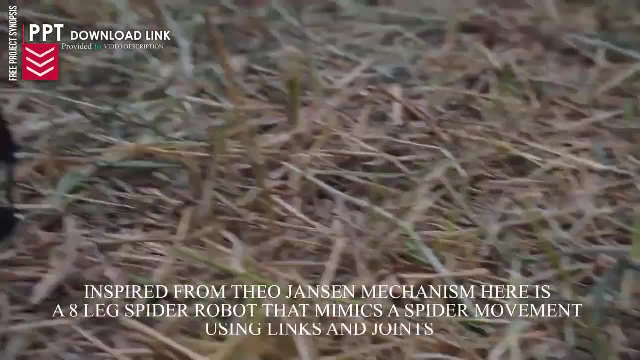 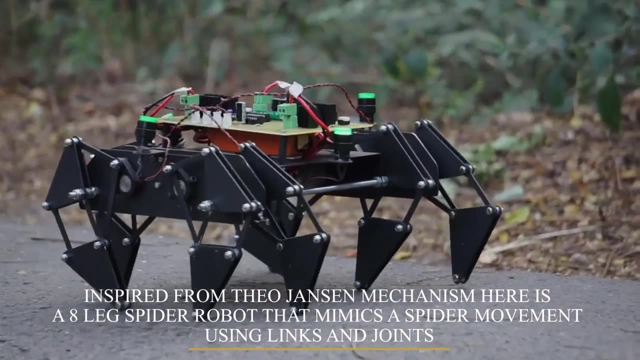 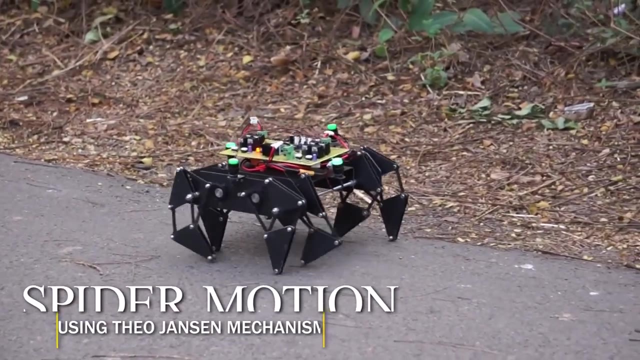 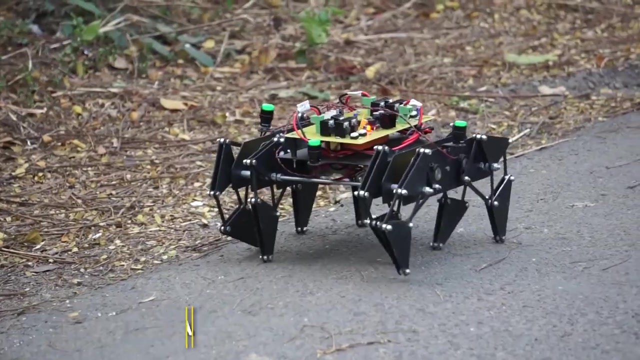 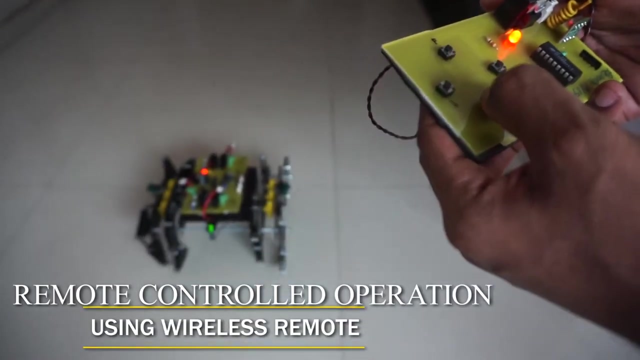 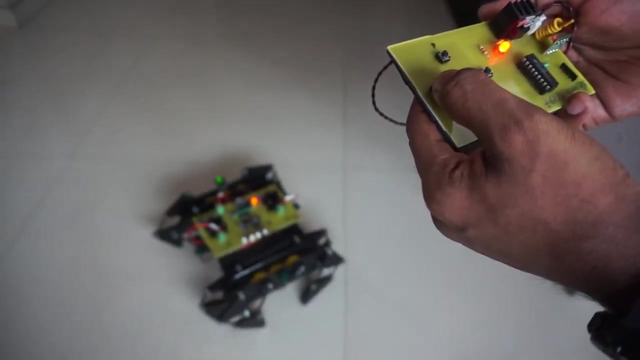 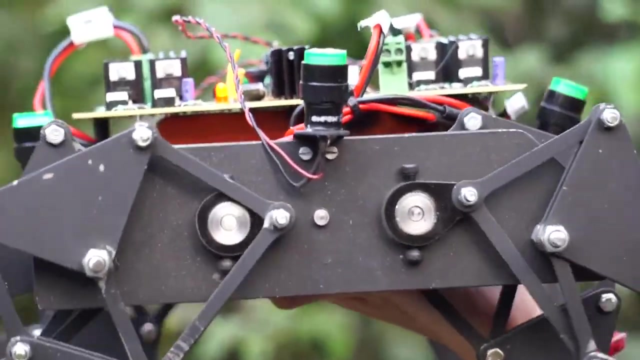 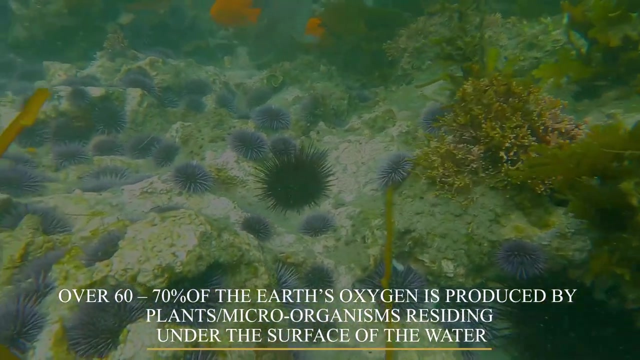 wheels over sand and rough terrain. Inspired from the Theo Jensen Mechanism, here is a 8-leg spider robot that mimics a spider movement using just links and joints. Thank you, Solar Lake Pool Cleaner. Over 60-70% of Earth's oxygen is produced by plants and microorganisms residing under the surface of water. 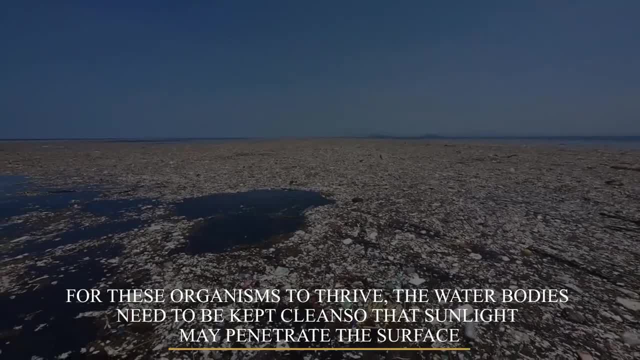 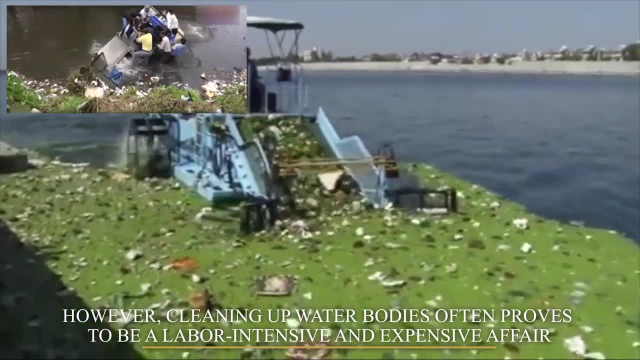 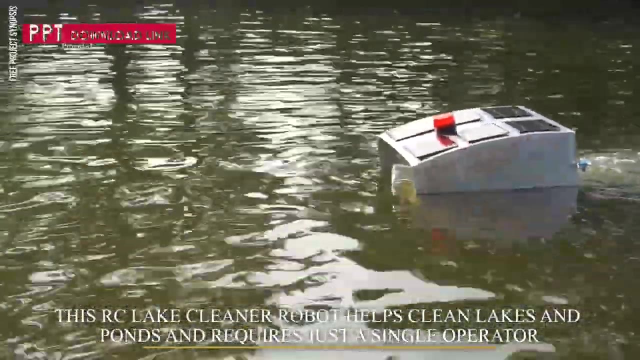 For these organisms to thrive, the water bodies need to be kept clean so that sunlight penetrates the surface. However, cleaning up water bodies often proves to be labor-intensive and an expensive affair. This RC Lake Cleaner robot helps clean lakes and ponds and requires just a single operator. 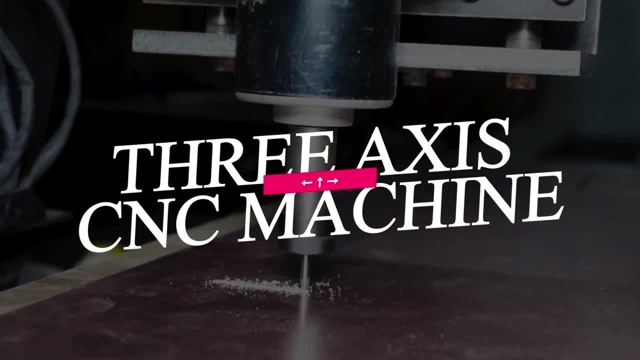 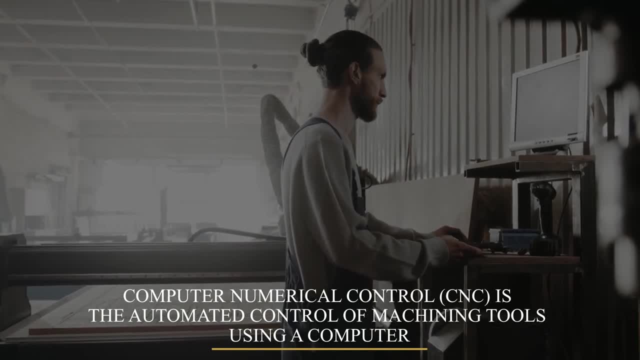 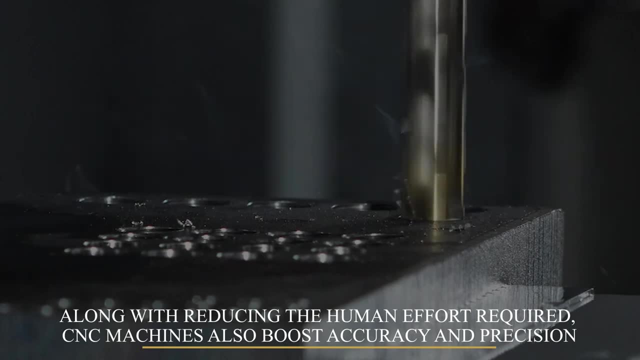 3-Axis CNC Machine- Computer Numerical Control. CNC is the automated control of machining tools using a computer. Along with reducing the human effort required, CNC machines also boost accuracy and precision. This 3-axis CNC machine uses an array of stepper motors for engraving and cutting. 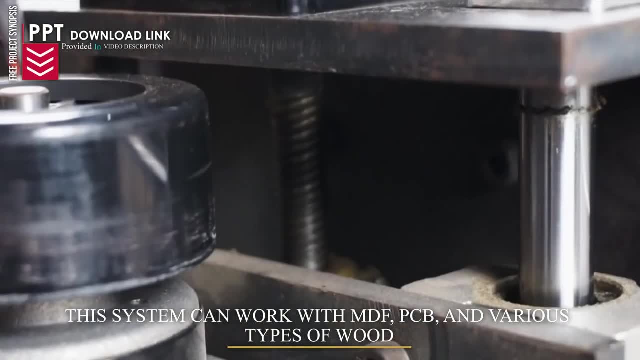 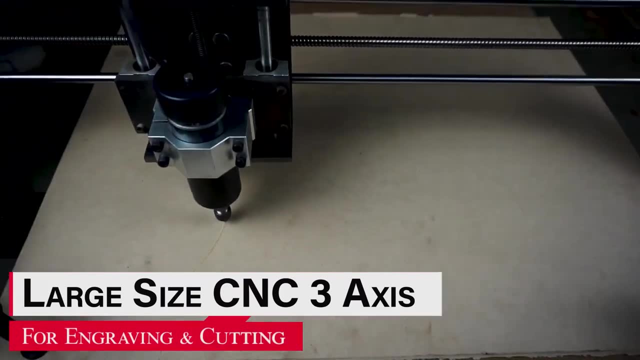 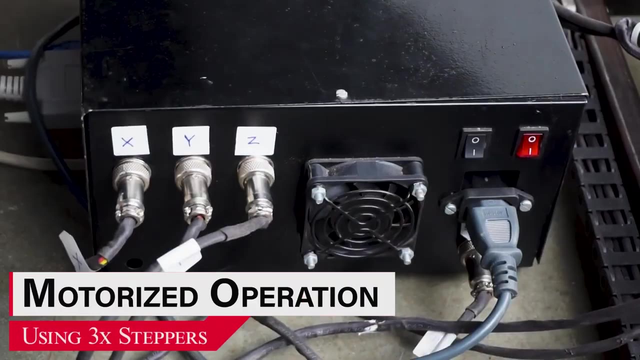 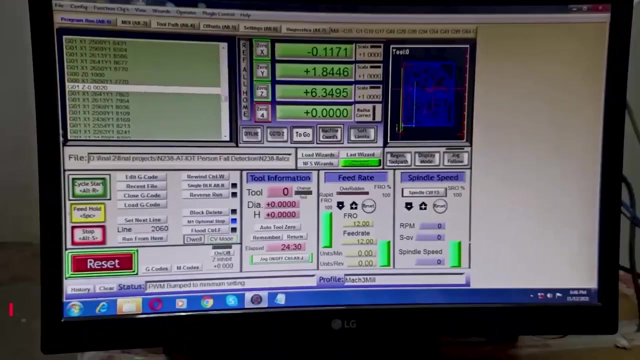 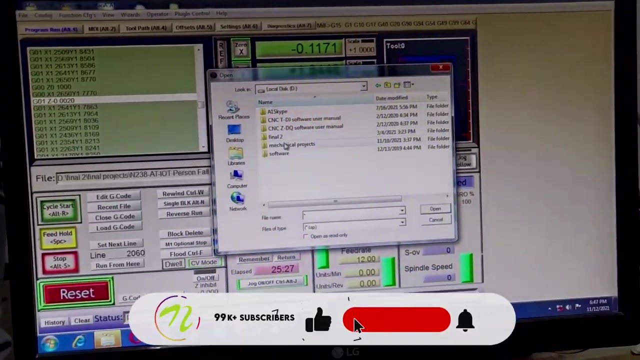 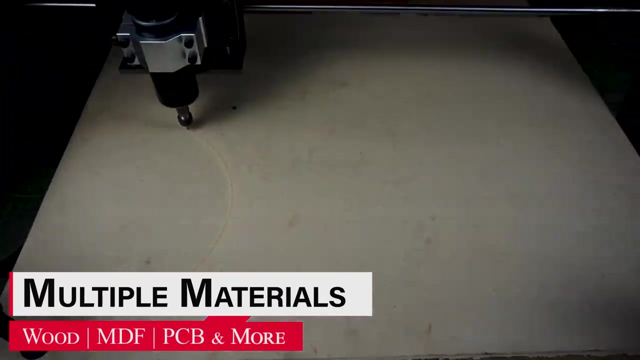 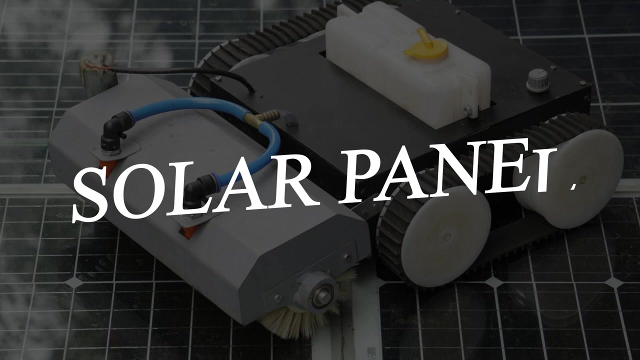 The system can work with MDF, PCB, Acrylic, as well as all types of wood. This machine can also China Rock, Silicone, Subtractable Camouflaging, movable seaming, Purifying, илли Solar Panel Cleaner Robot, Along with being non-polluting solar energy. 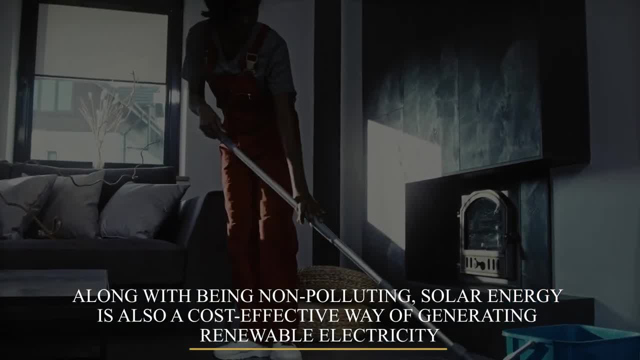 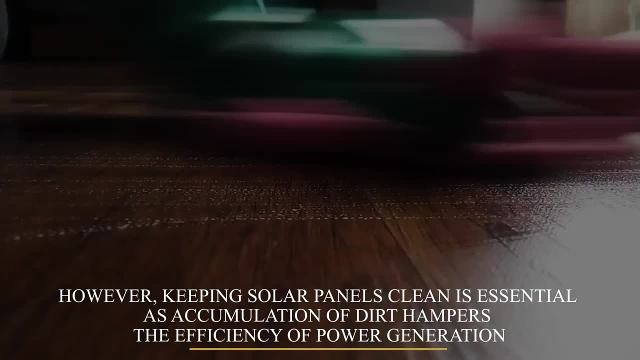 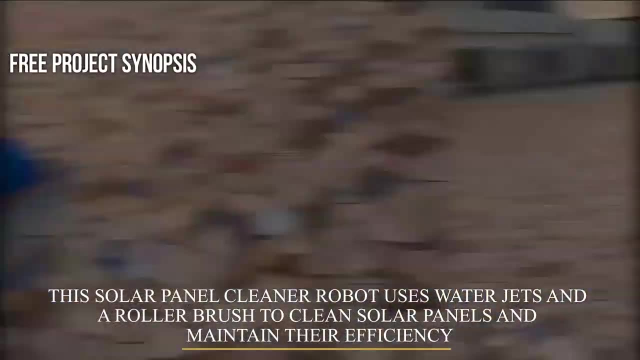 is also a cost-effective way of generating renewable electricity. However, keeping solar panels clean is essential, as accumulation of dust hampers the efficiency of power generation. Although manually cleaning solar panels can be tedious and hazardous, This solar panel cleaner robot uses water jets and a roller brush to clean solar panels. 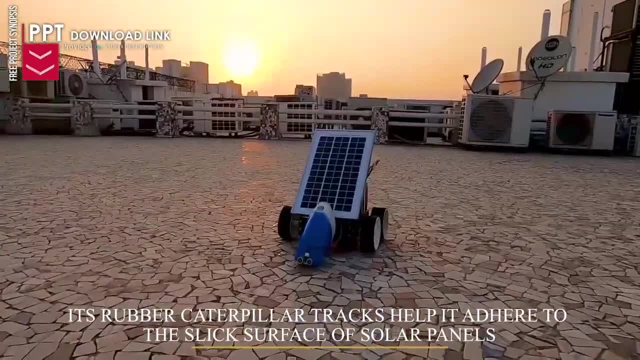 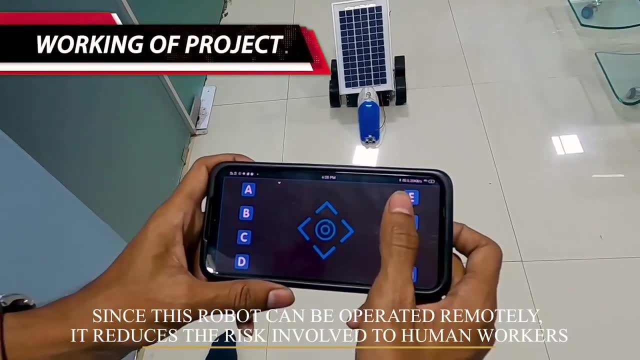 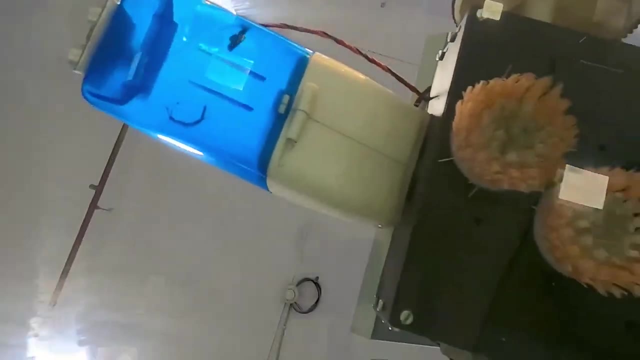 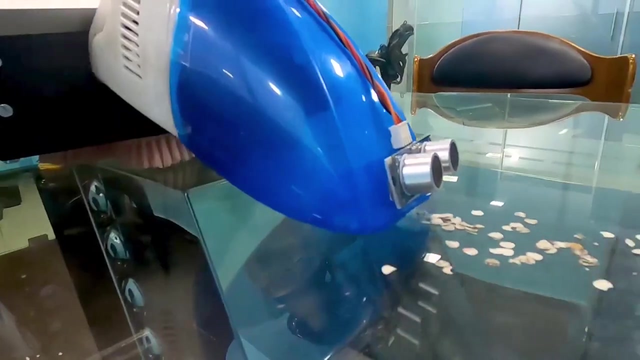 and maintain their efficiency. Its rubber caterpillar tracks help it adhere to the slick surface of solar panels. Since this robot can be operated remotely, it reduces the risk involved in using human labors. It can also handlemund water taps and all Composed Mmm. I. 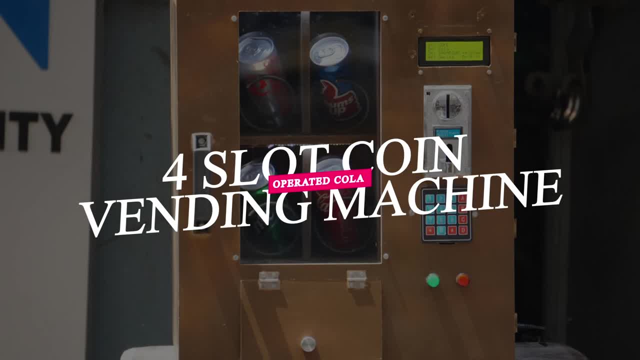 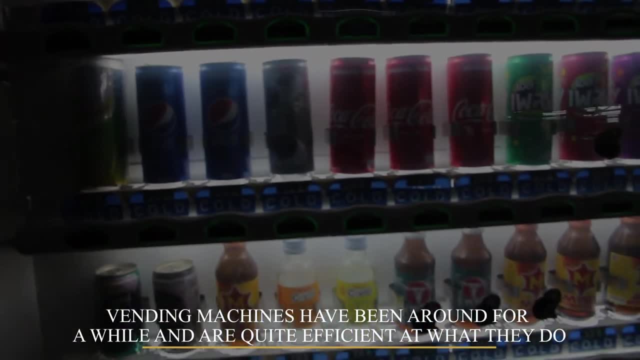 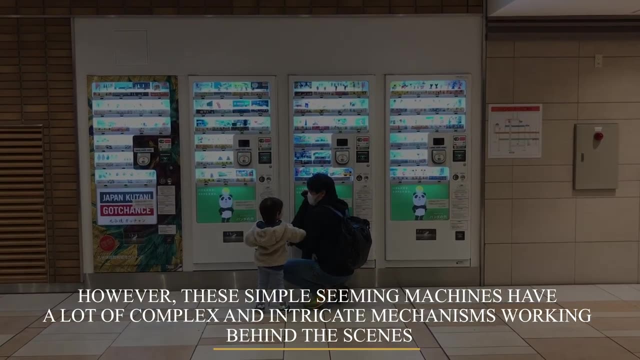 4-slot coin operated Cola Vending Machine. Vending machines have been around for quite a while and are quite efficient at what they do. However, these simple seeming machines have a lot of complex and intricate mechanisms behind the scenes that they have to care about right.